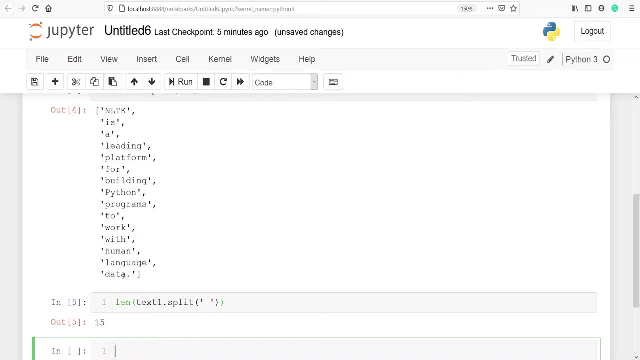 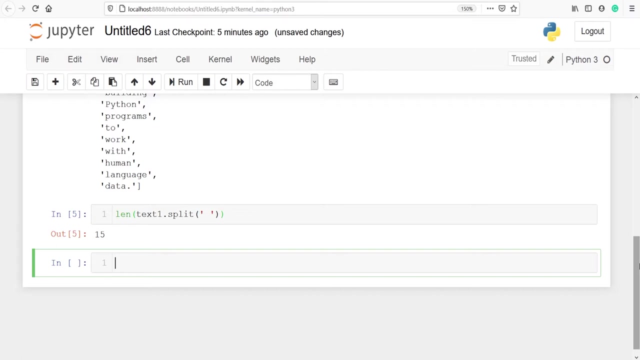 this is not correct. we should not get full stop here, because we are splitting words and full stop is not a word, so it should not come with word, it has to come separately. for that we are going to use the inbuilt function of nltk and the inbuilt function is tokenization from nltk. i will call the. 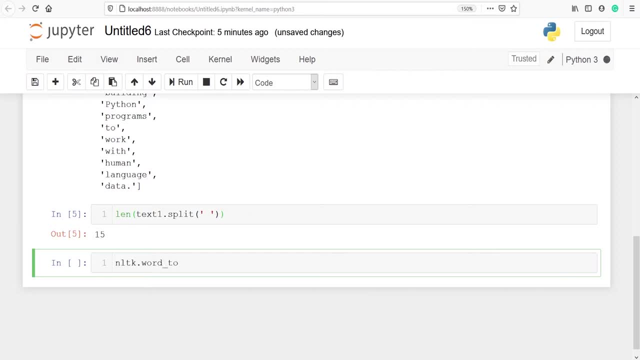 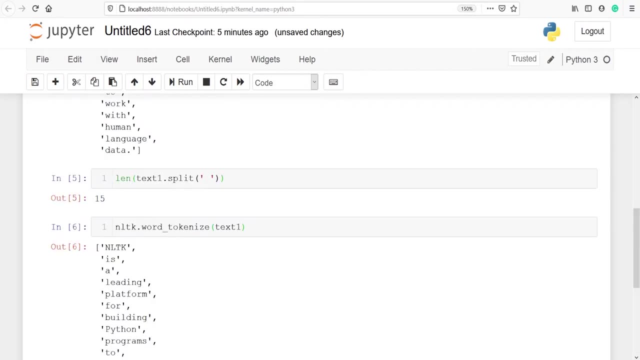 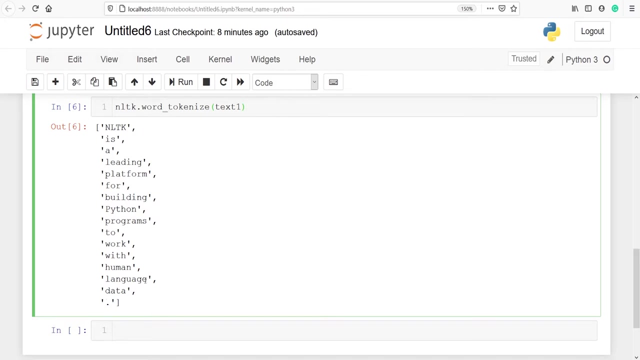 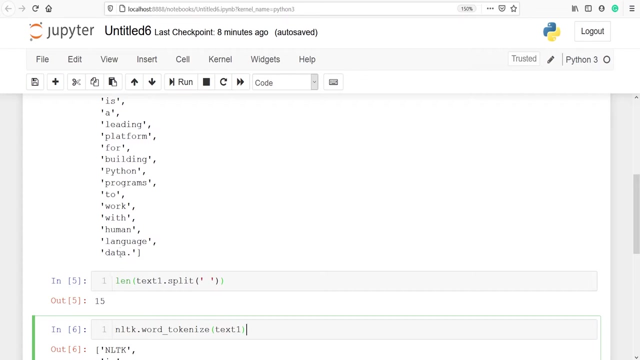 method: word underscore: tokenize. and now i will pass the variable text one. let's execute our code. in the output you can see that we got all the words here and here we got full stop as a separate word. but if we compare it with the above example, you will see here we got full stop along with the word data, and the total number of words are 15. 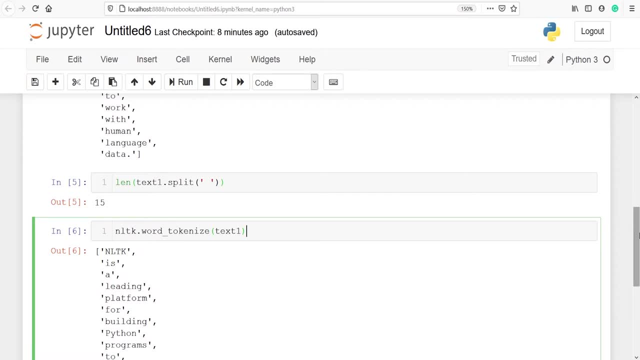 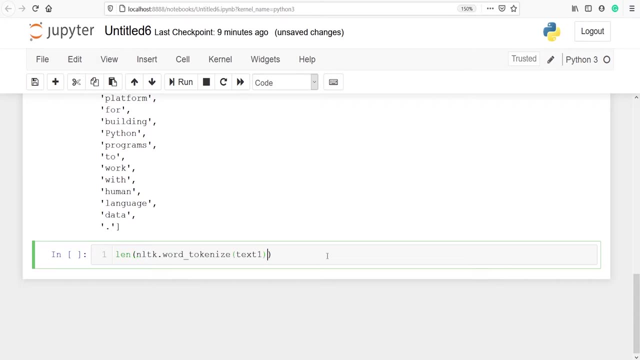 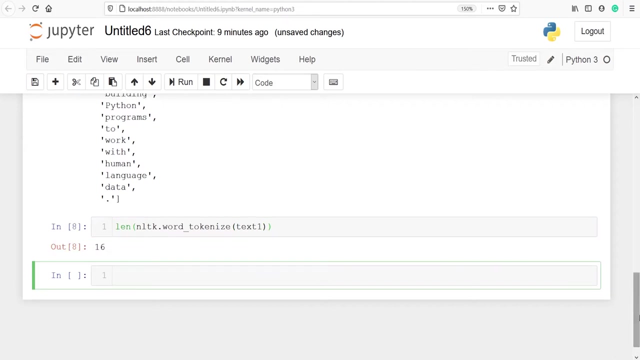 let's copy this code. let's use the length method length and paste the code, and we should get 16 now because we got one more word here, full stop. let's execute our code. in the output you can see that we got 16 here earlier. the count of words. 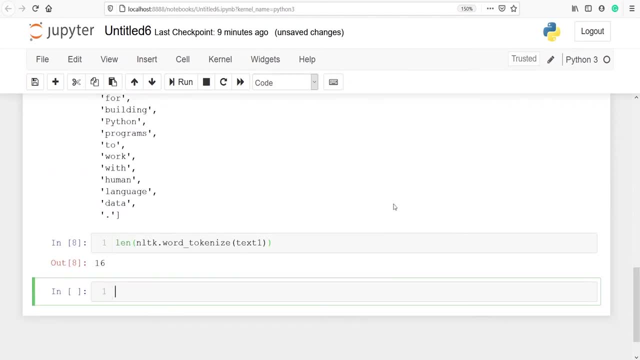 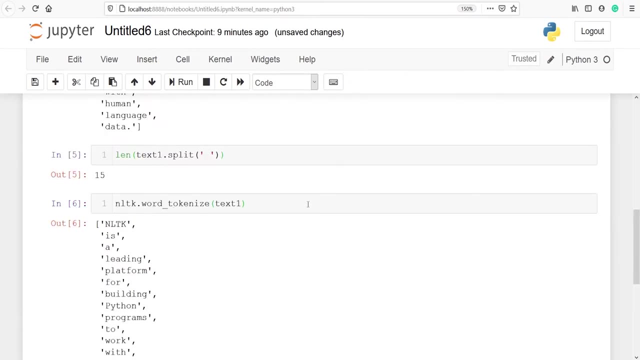 verb 15 and now the count of words are 16, because this full stop is now a separate word. when you use this inbuilt method, tokenize, it performs very well, so you should always use this inbuilt method verb underscore, tokenize to tokenize your words instead of splitting. 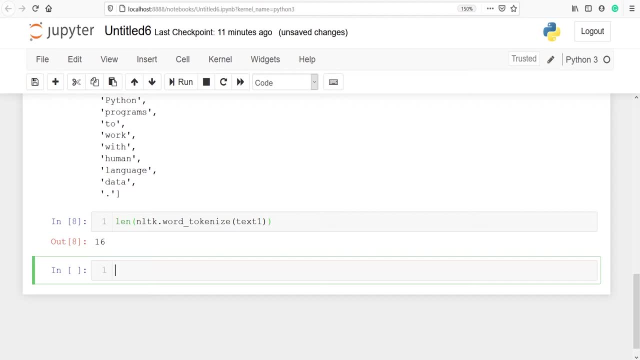 on space. next we will learn about sentence split. what is a sentence? what is a sentence boundary? we need to know this because we have to split sentences from a long text. let's write a sentence and save it in a variable. i'll make one variable, text2, and i'll save. 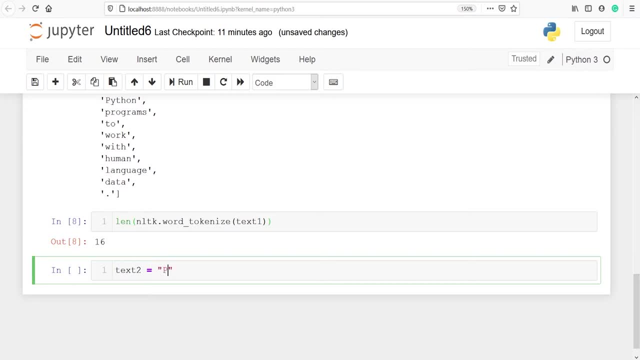 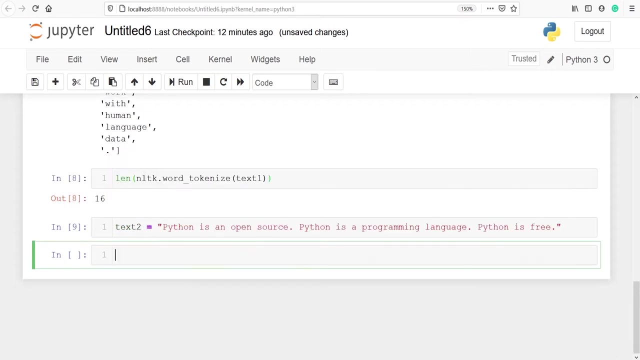 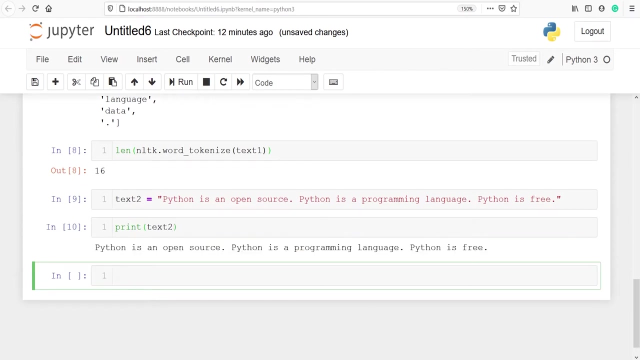 some sentences. first is: python is an open source. next is python is a programming language. next is: python is a programming language and the third sentence is: python is free. let's execute our code, let's print our variable text2. we already know a sentence end with a full stop or a question mark or an exclamation. 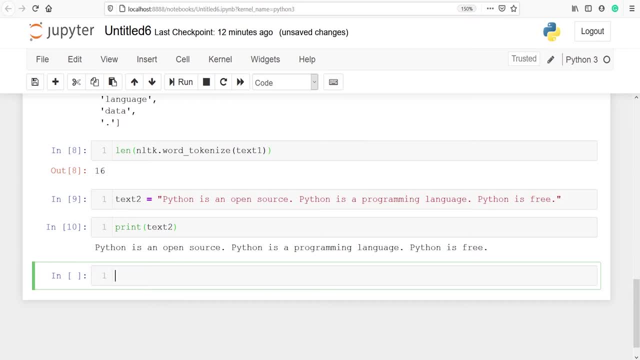 mark and so on. we you already know a sentence end with a full stop or a question mark or an exclamation mark and so on, sentences, and these are: python is an open source, python is a programming language. python is free total. there are three sentences. let's use inbuilt function of nltk to find the number of sentence. 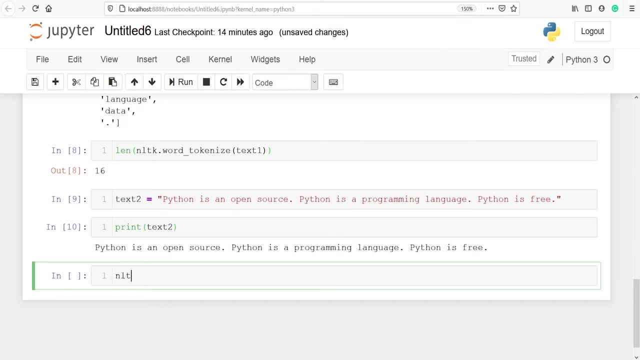 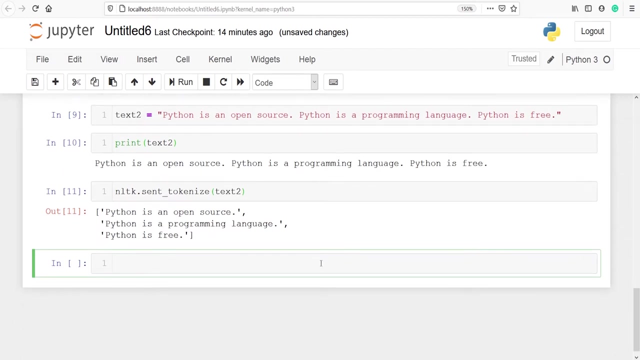 in a text from nltk. let's call send, underscore, tokenize, and then we will pass our variable text to. in the output you can see that we got three sentences here. the first is python is an open source, the second is python is a programming language and the third is python is free. 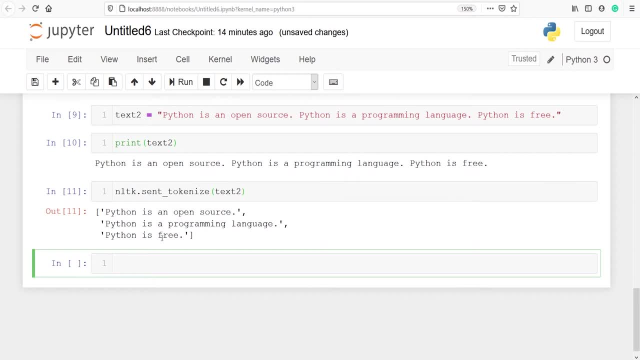 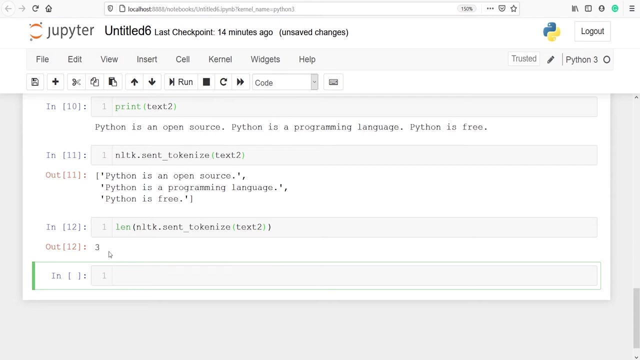 and to get it into number we will use the method length. i'll copy this code from here. i will call the method length and inside this i will paste the code. let's execute our code. in the output you can see that we got three year because there are total three sentences in our text. text two: 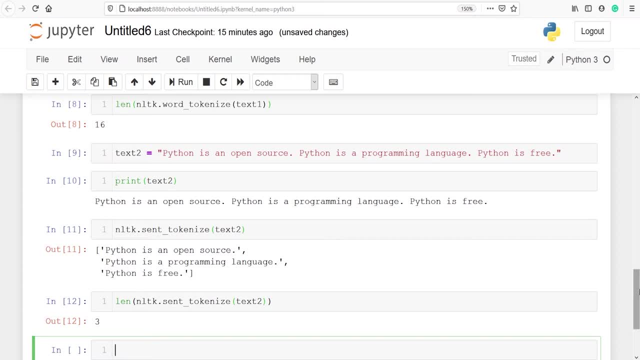 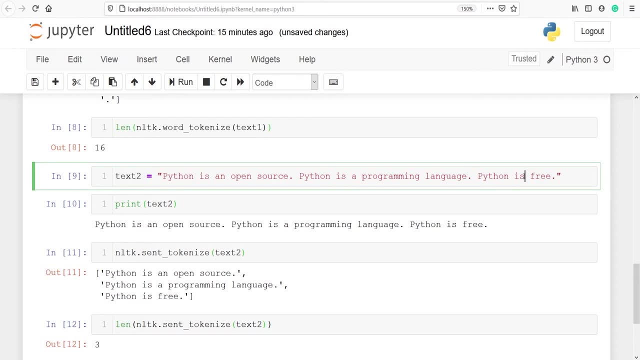 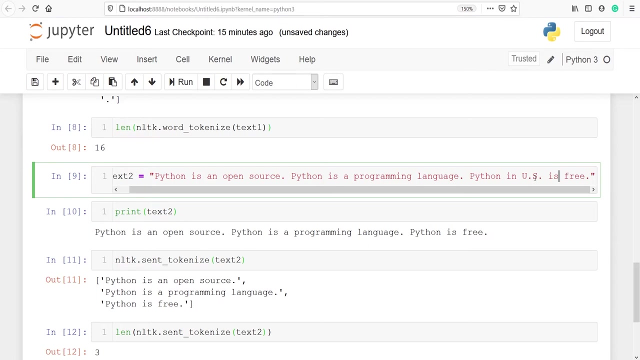 this is how you can extract number of sentences from a text, and if i'm put here, python is python in us is free. now you will see that we have a full stop here twice. we have a full stop here here, also us, and we also have a full stop here after free. if I execute this code, I'll 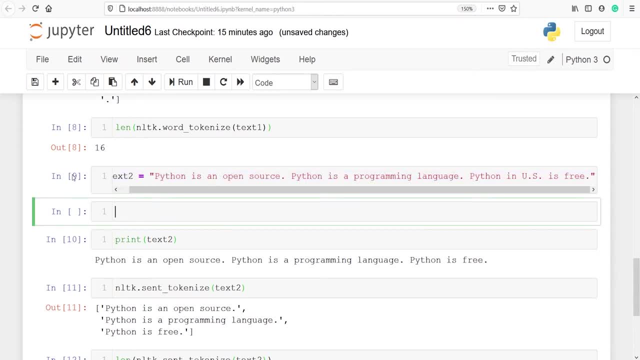 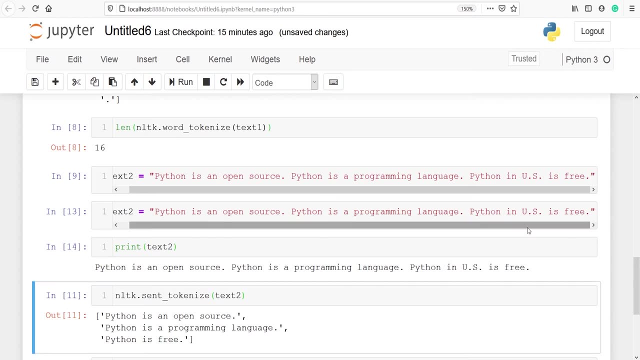 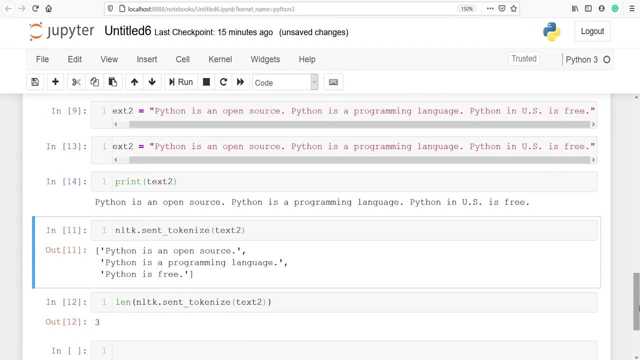 just copy this code and then I will paste it here. now let's execute our code. if I run this and print it, you will see we got. python is an open source. python is a programming language. python in us is free. now how many sentence we will get? because after every full 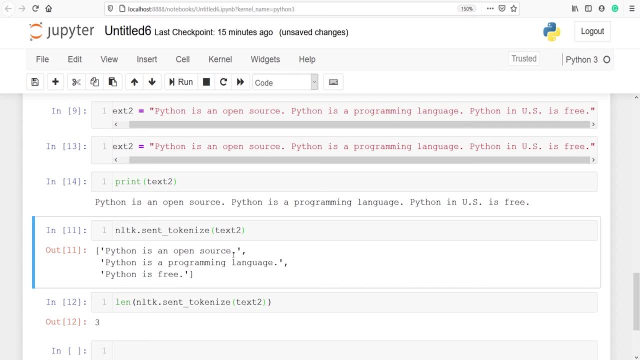 stop. we are getting a new sentence here. we will see. after every full stop we are getting a new sentence and now we got a full stop in us. so do you think we will get four or we will still get three? let's execute our code and see. in the output you can see we.